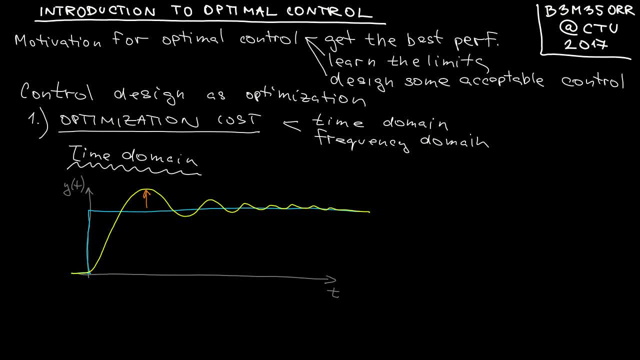 identify here the overshoot, which is a good candidate for minimization. or we may want to minimize the rise time, or we may want to minimize the settling time. the trouble with all these indicators is that each one of them only covers one particular aspect. so, in case you want to minimize the rise time, what could? 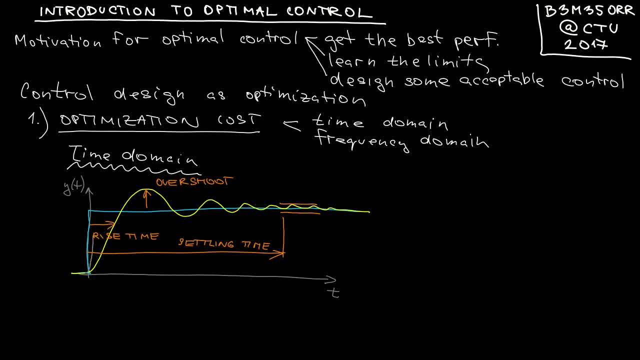 happen is that you will significantly deteriorate the overshoot and the other way around. if you want to minimize the overshoot, you will get very sluggish response and very large rise time. now, of course, you can always handle this by imposing constraints on the other characteristics, or you can what you can. 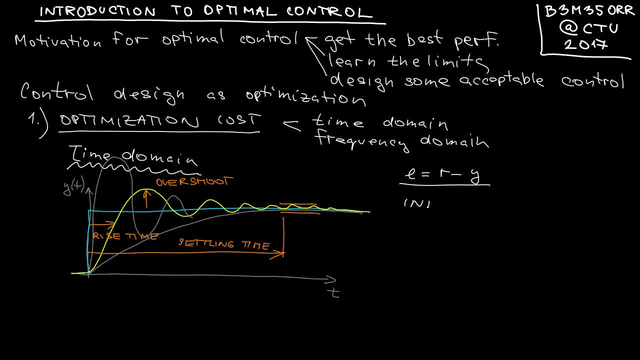 also do is that you can use the so-called integral criteria. after defining the regulation errors e, e, you can define your optimization criterion as the integral of absolute value of error or integral of time, weighted absolute value of the error or integral of squared error. these are even given some names in the literature, such 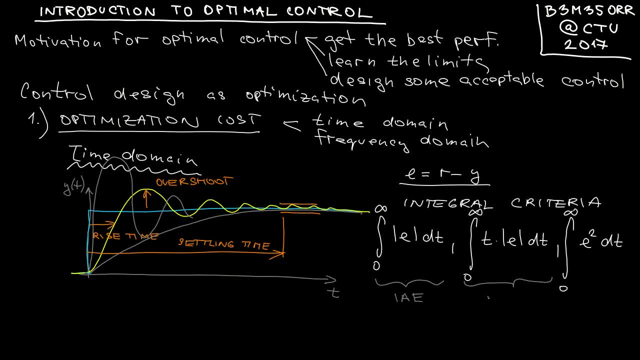 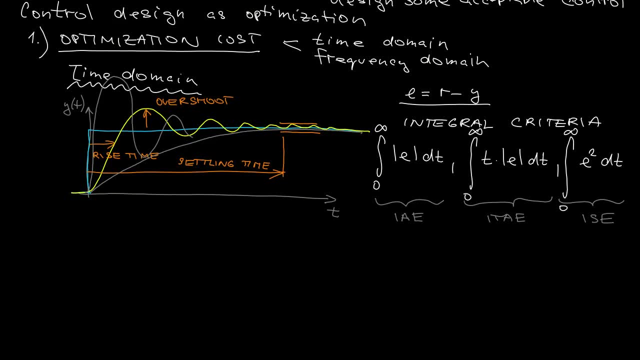 as integral of absolute error, integral of time times absolute error and integral of squared error. now, all these criteria only handle performance. you can, of course, include the control aspects in constraints, or you can include them directly in the optimization criterion, and thus realizing the trade-off between performance and control effort. the most popular among these is apparently or the. 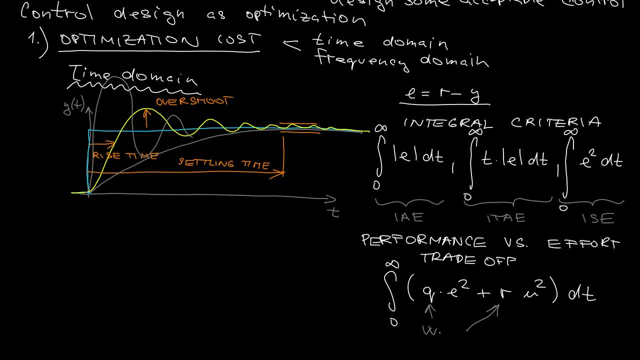 most popular is simply the one that you can see here, where Q and R are parameters which you use to express different preferences for the error in E and the error and effort berg moduler for the error in d, since A and I actually also use the 0 to. 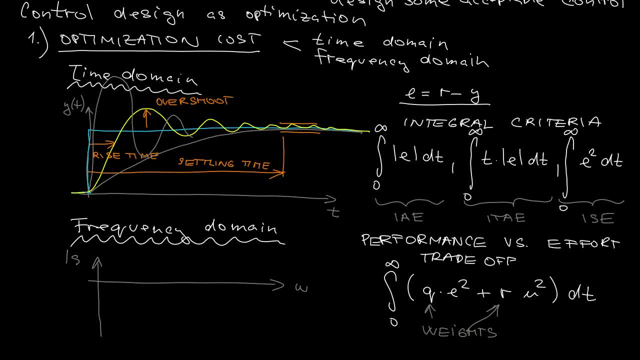 b, Q and E. this area is also very particular for the level of registration or measurement, so you could basically just write a value that thisggi is actually satisfied by itself does not mean you're not almost satisfied because the error is have to the limit, and it also means that you have to spit it out so that it area. 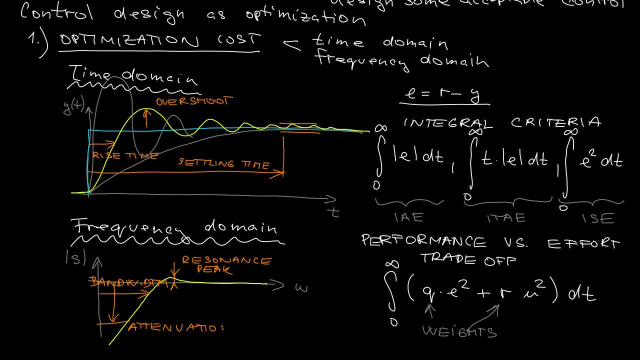 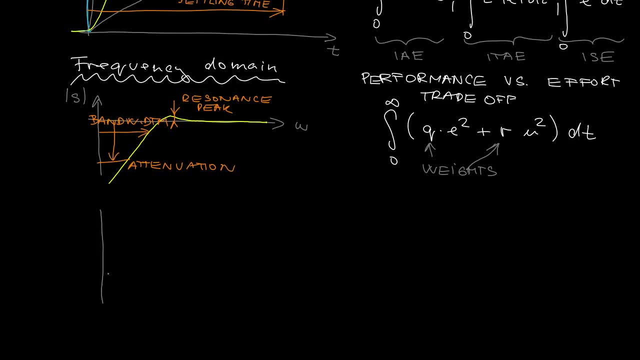 as before holds here, in that these individual characteristic only cover one particular aspect. so if you want to now express something more more global, you can do it by introducing frequency by frequency constraints on on these frequency responses. for instance, this upper bound on closed-loop sensitivity function, we will label it as 1 over W and then the resulting closed-loop. 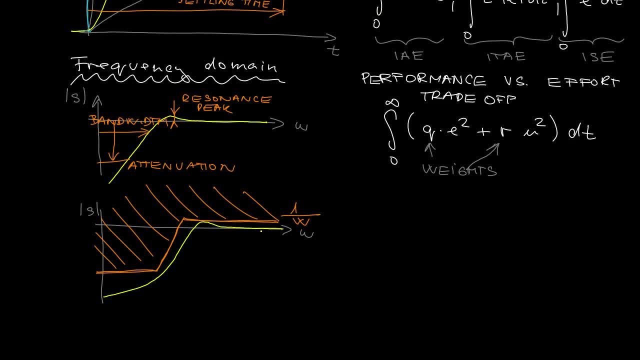 transfer function, sensitivity function should look like this. now you can verify by yourself that the this visually depicted condition can be expressed as the condition that supremum over all frequencies, from magnitude, frequency response of W times s should be less than 1, which makes it a perfect. 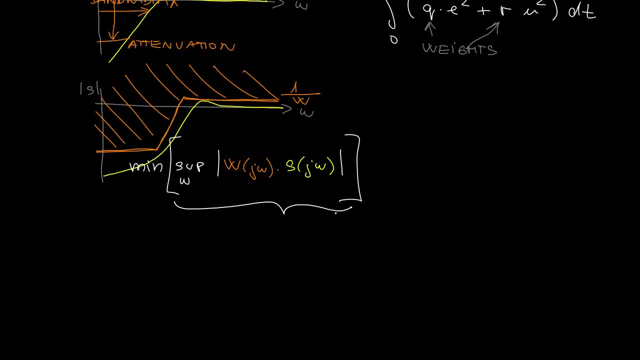 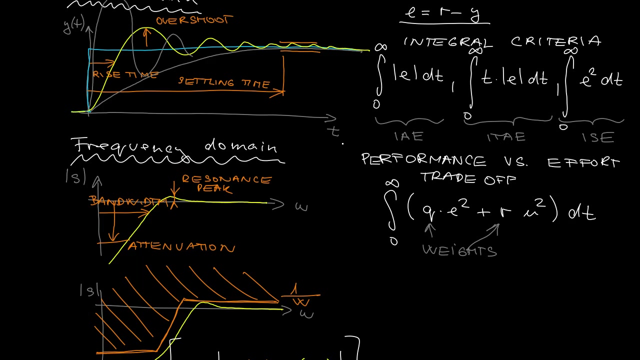 candidate for minimization. by the way, this candidate for minimization is also compactly labeled as H infinity norm of W times s a name, and this is called H infinity norm of the system, and in fact the concept of norm can also be identified here in the time domain, where 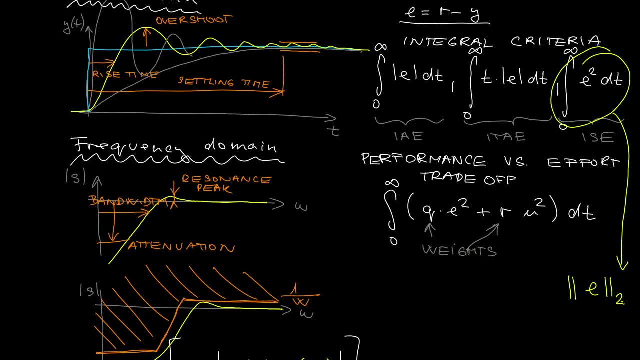 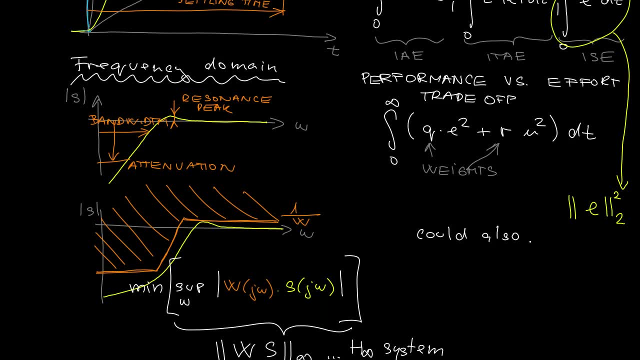 for instance, the integral of square of the error can be seen to be the squared to norm of the signal, or similarly, the integral of absolute error can be compactly labeled as one norm of the error signal and in fact the concept of norm can also be identified in time. 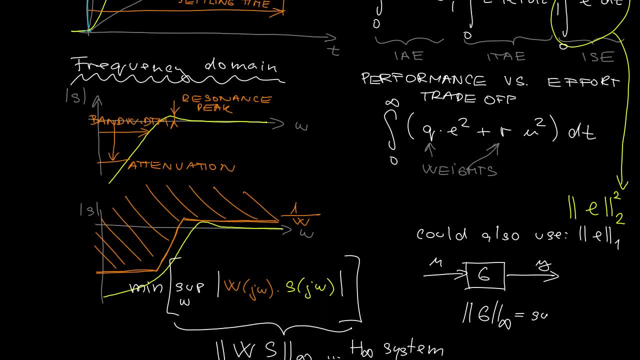 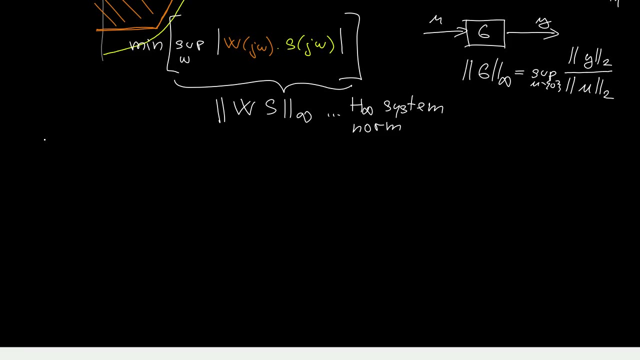 domain. for instance, by considering input U, output Y, the H infinity norm can be shown to be seen as worst-case gain of two norm of the in output with respect to the two norm of the input, but more on system norms later in the course. the other question that needs to be answered in order to use optimization as a 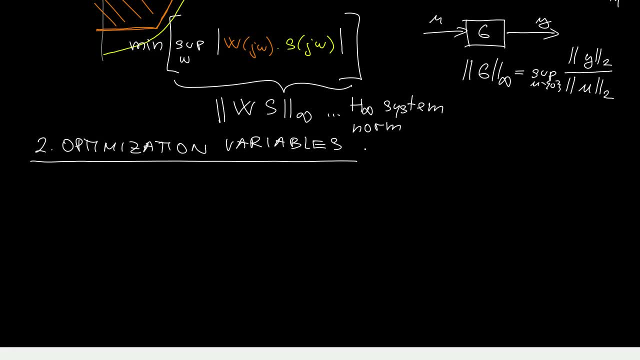 procedure for control design is what will be the optimization variables. there are two options: either we will optimize over controllers or we will optimize over control signals. with the optimization over controllers we are running into troubles if we do not make any restriction here, because the problem is then intractable. so we typically need 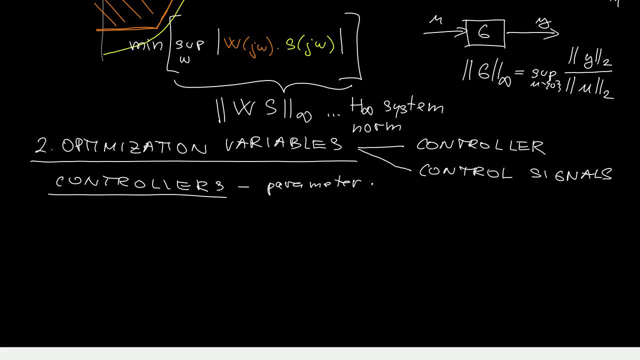 to fix the structure, and then we do optimization over the controller parameters, such as coefficients of a PID controller. there are two major issues here. one of them is that first you will need to express the optimization criterion, which we will label as J in the course, you will need to express it as a function of the optimization variables PID and. 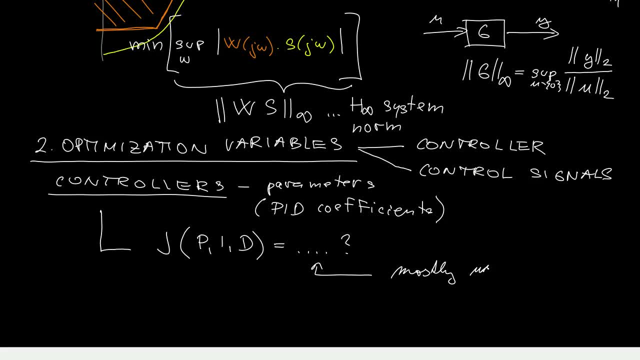 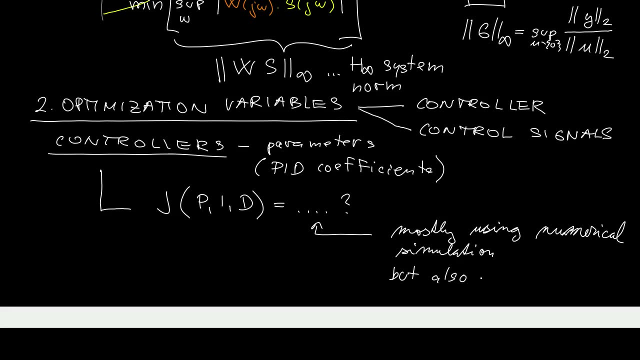 typically, with the exception of very simplest linear systems, you cannot do it analytically. you will have to resort to numerical simulation, with all the unpleasant consequences, such as troubles to evaluate the first and second derivatives. there is a relatively recent contribution to this domain by means of so-called algorithmic differentiation, which 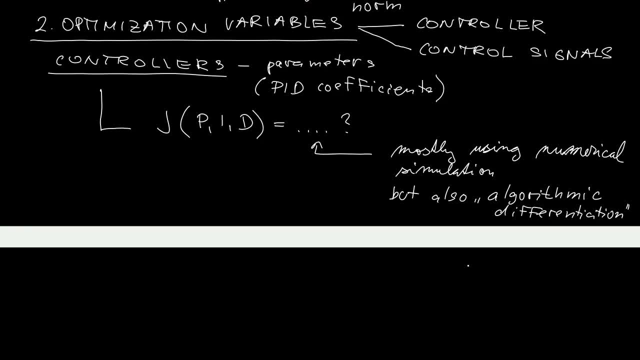 handles, which can handle this, but we will not cover it in this course, so look it up on your own then. the other issue here is more serious, and that is that if you only want to minimize this or that characteristic, this is not enough. you will also have to impose additional constraint here, and that is closed-loop. 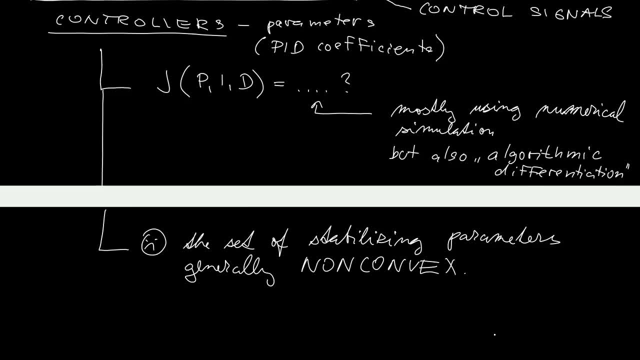 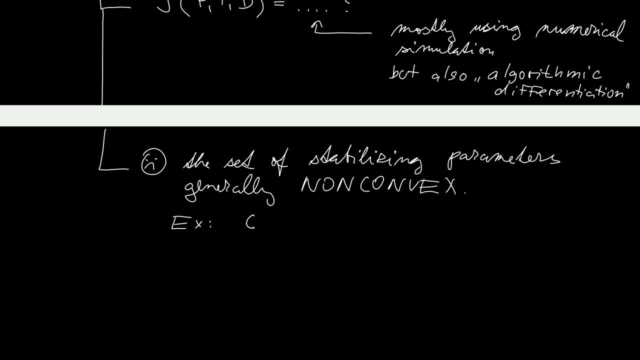 stability, and the trouble is that the set of stabilizing parameters of the controllers is typically non-convex, which renders the optimization difficult. consider even just a linear system, say system described by transfer function G, with the denominator polynomial of the third degree. in order to check its stability, you may invoke: 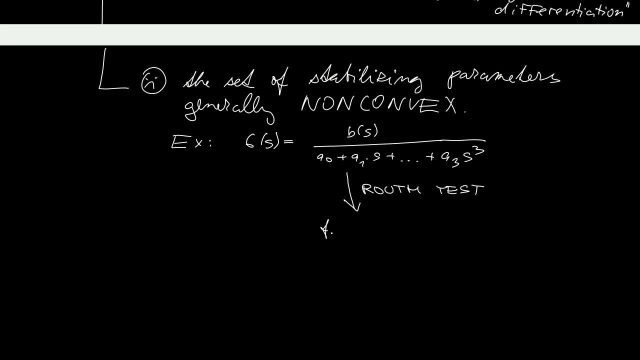 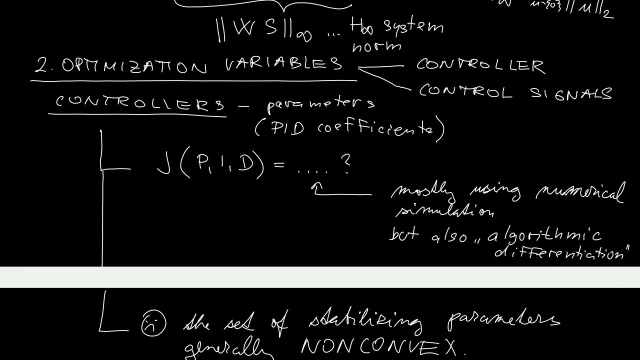 Routh test which will give you a few functions and which will be functions of the of the coefficients of the system, and these functions will give you a set of inequalities. these will be typically these: F functions will be typically nonlinear functions of of the parameters of the system, hence also parameters of the controller, hence, and typically these: 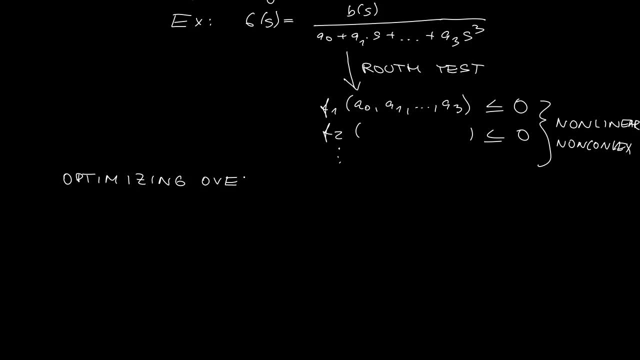 constraints will be non-convex. so enough for enough for optimization over control parameters, and let's now discuss briefly optimization over control signals. in the time domain, the control signals are essentially functions. that means you will have to optimize over signals, which is something for which are not yet ready, however, in